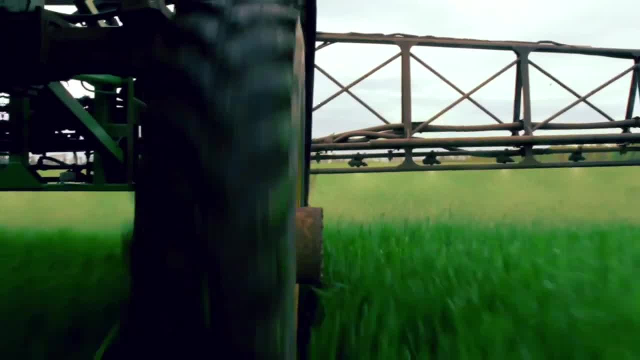 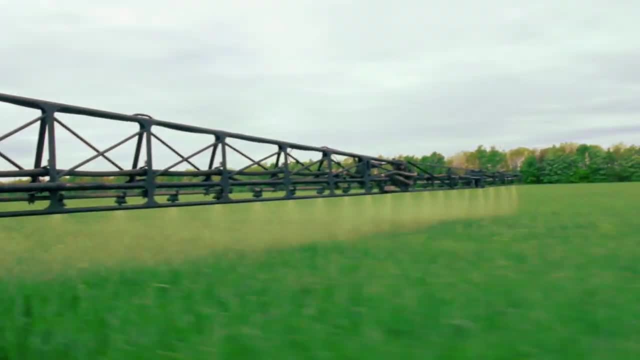 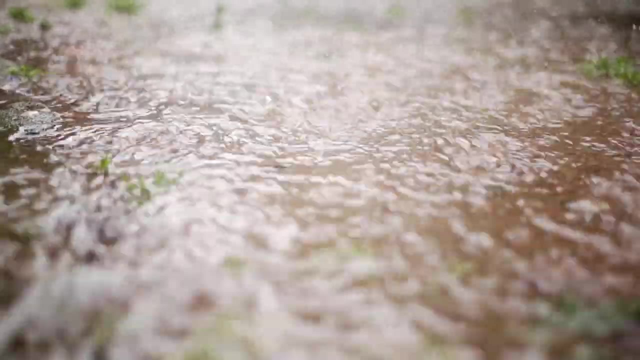 they grow the maximum amount of product they can, So they add fertilisers to their crops to increase production. These fertilisers are important in meeting global demand for food, But sometimes there's a problem: The fertilisers added to farmland can get washed away by over-watering or heavy rain. 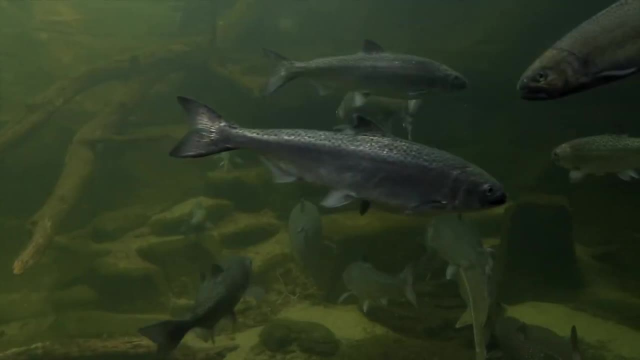 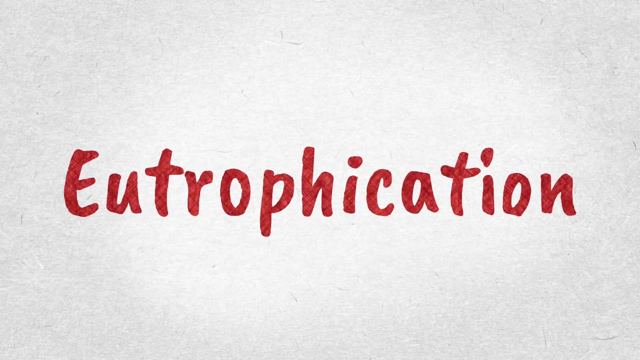 When they get washed into lakes and oceans. it's bad news for a lot of species that live there. So what can we do? Utilisation of water. Utilisation literally means well-nourished, because it happens when a body of water becomes. 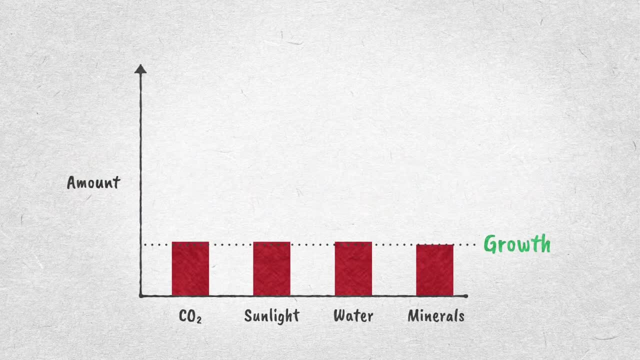 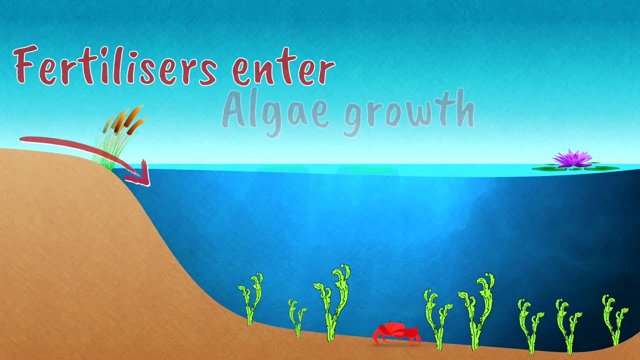 enriched in dissolved nutrients. Minerals are usually a limiting factor for growth of producers in water, so when minerals from fertilisers enter the water, this is great news for the photosynthetic algae, which grow in number. Algae grow as a layer on top of 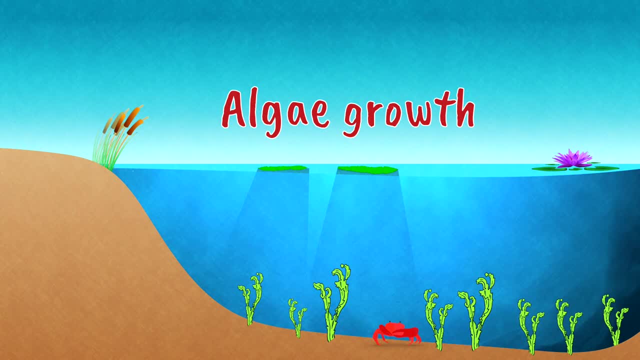 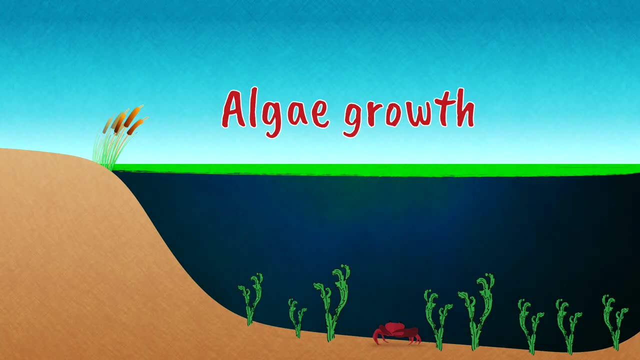 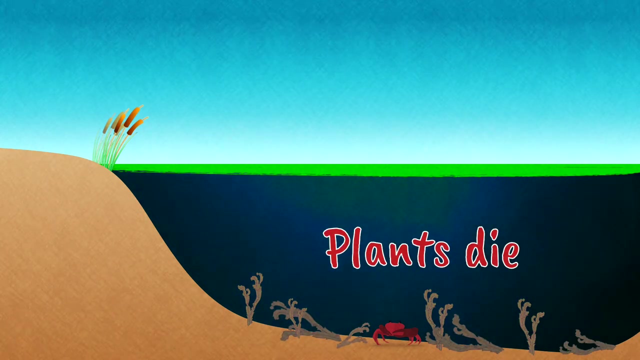 the water. After a while, the algal growth becomes so extensive that it's hard to cover the surface. This is where things start to go bad. Very little light can pass through this surface layer, so eventually the plants at the bottom die from a lack of sunlight. 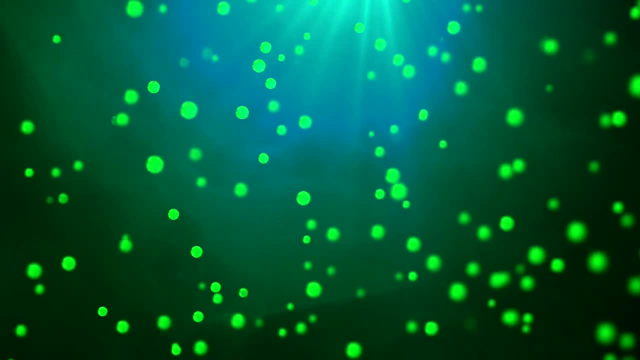 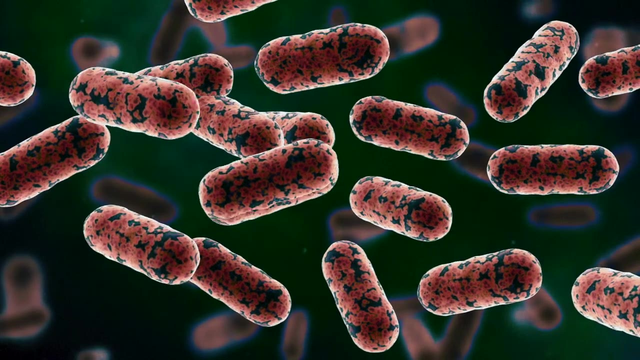 As part of their natural life cycle, algae die and are replaced by more algae, And this provides lots of organic matter for microorganisms to decompose. These microorganisms rely on aerobic respiration, Meaning that in addition to the food they take, they also have the 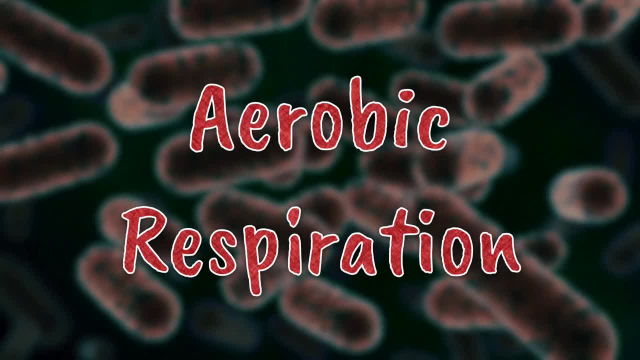 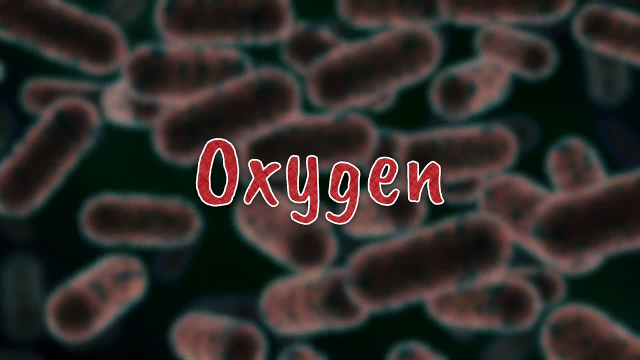 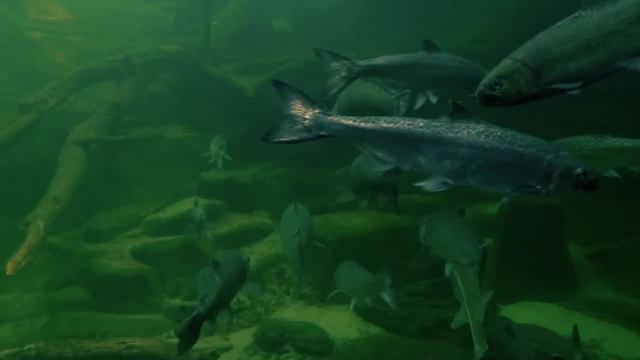 ability to decompose. So what can we do? In addition to the food they take in, they also require oxygen. With such an extensive supply of dead organic material as food, these microorganisms grow in number and deplete the oxygen levels in the water. Fish and other organisms living in the water also rely on 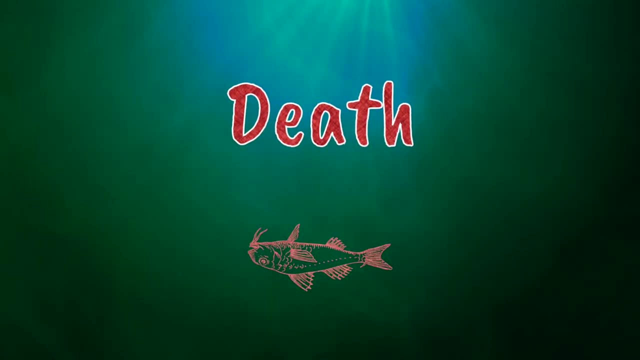 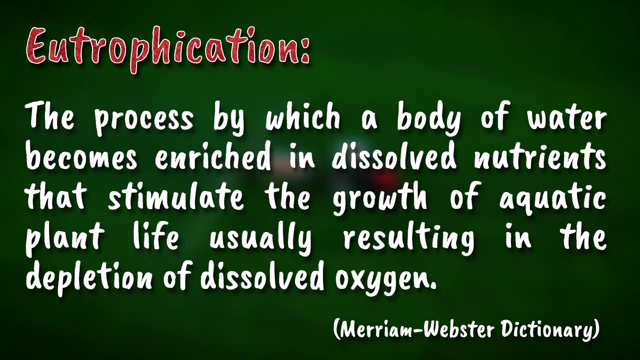 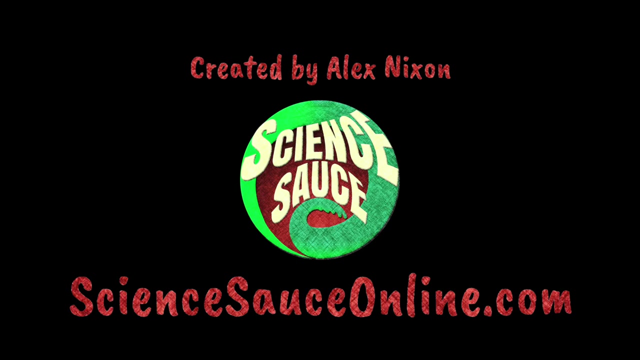 this oxygen, and when it becomes depleted, it results in death and a reduction in biodiversity. In addition to the food they take in, they also require oxygen. So what can we do?